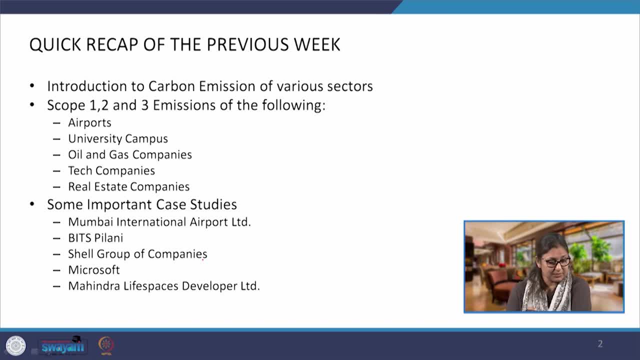 the efficiency and reduction of emissions is concerned. Then we looked at Bitspilani campus, we looked at Shell group of companies, we looked at Microsoft and Mahindra Lifespaces Developer Limited. When we saw their scope, 1, 2 and 3 emissions, we actually looked at the numbers. 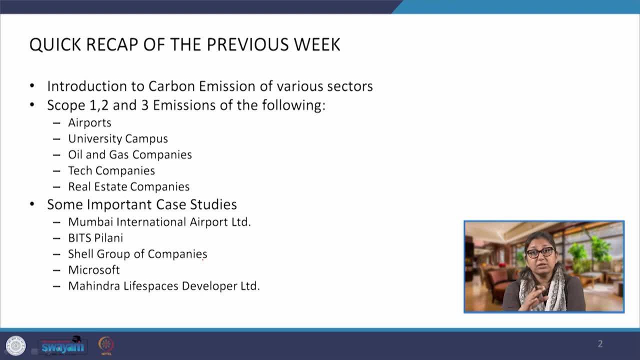 as given in their publicly available audited and reported reports. So these case studies were actually through the commitments and also the audited reports that these companies have provided in public forum. So this is what we understood Now, also when we were discussing about each of these different 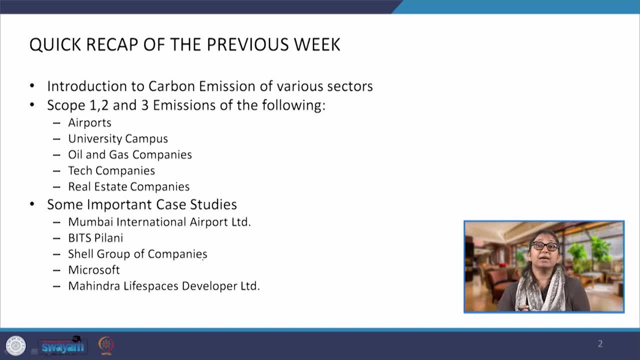 types of companies and sectors. we saw that building design and construction plays a significant role in reducing the GHG emissions- One towards emissions and also towards reducing the GHG emissions- and there is a wide scope of doing so. Another thing that we understood as a takeaway from this entire discussion was that the primary 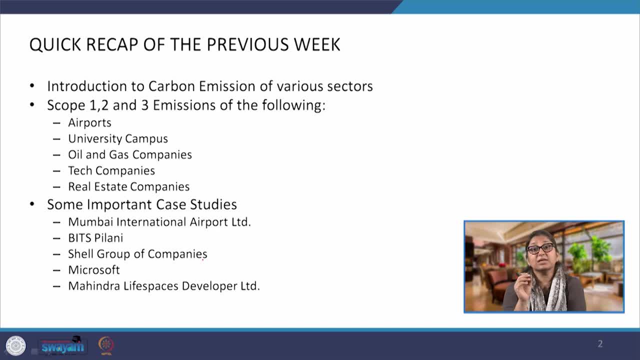 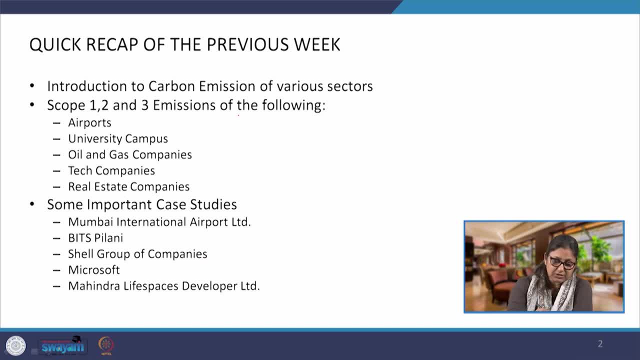 acoustic comfort and for these different variety of functions that we saw. whether it is an airport building or a university campus or a tech company or anything, The primary purpose of buildings is to reduce the extremity of the climate, of the weather around and to provide a comfortable. environment And, if you see, cannot go inside, as that is also not actually united with housing. So these are just some examples, So I forgive you for these. So these are just some compounding advantages that we saw withอน wathings. I hope that covening健ân silently rented collaboration. 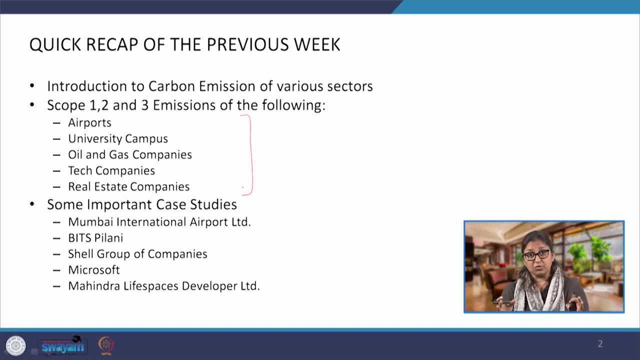 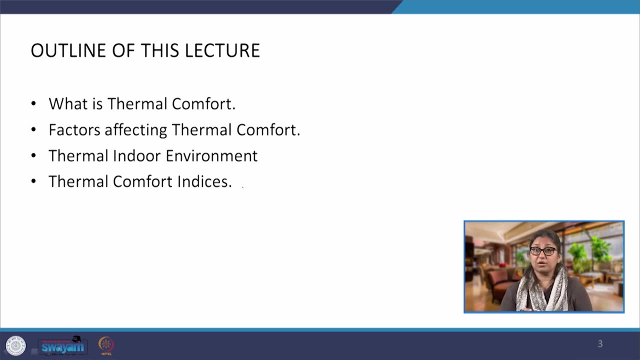 inside, And in that process of doing so, of providing a comfortable environment, a lot of energy is consumed during the operations of the building. So at the end of the day, we are talking about providing comfort. Now, in this particular lecture, we are going to talk about thermal comfort. 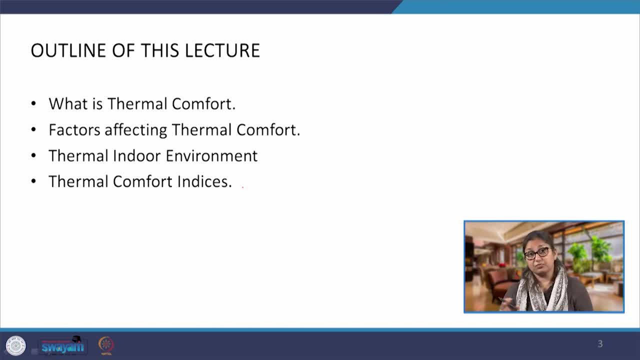 first There is going to be other dimensions: visual comfort, acoustic comfort. we are not going to cover as part of this course, but we will very briefly understand the visual comfort and how it is ensured and how we can reduce energy consumption and emissions through that. But here we are going. 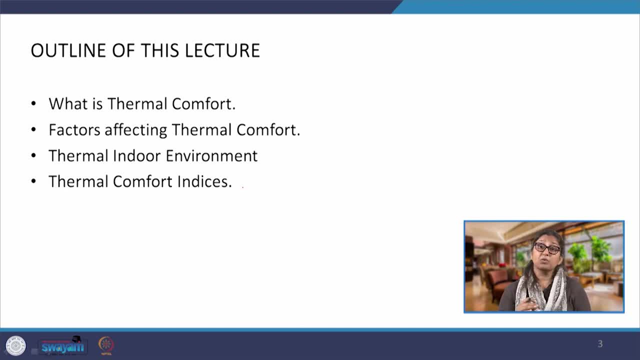 to quickly understand about thermal comfort: what are the factors which affect thermal comfort, the thermal comfort, thermal indoor environment, And we will look at not really thermal comfort indices, but we will understand that how thermal comfort can be created and how it can be used to create a comfortable environment, And we will look at not really 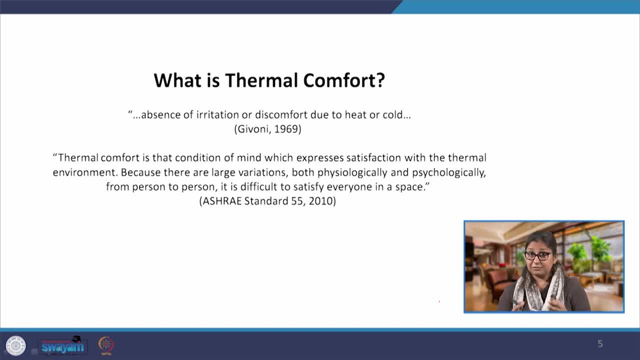 and understood as a concept So quickly. if we look at the definition of thermal comfort, it is the condition of mind which expresses satisfaction with the thermal environment. Because there are large variations, both physiologically and psychologically, from person to person. it is difficult to satisfy everyone in a space. Now it is basically the absence of irritation or 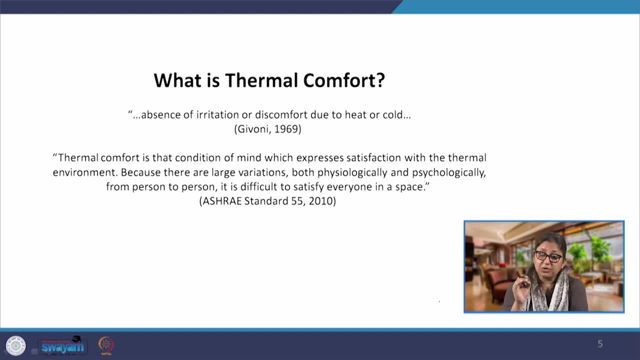 discomfort due to heat or cold is what we know as thermal comfort. Very simply, if I am comfortable right now, if my body does not need to exchange with the environment, the heat or cold, to maintain its comfort, that is when I will say that I am thermally comfortable. 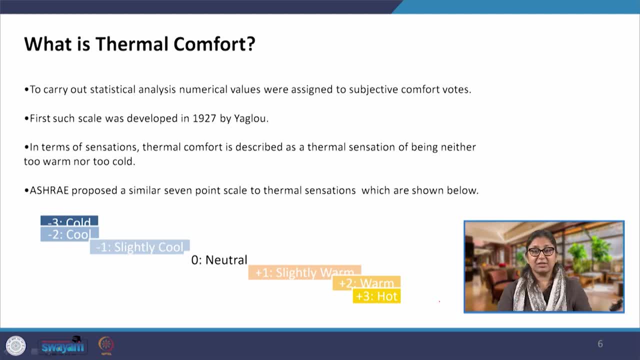 Now, how would we know that it is thermally comfortable? as we just saw that from person to person the perception will vary. So the scientists have worked towards it and they have developed something called thermal comfort indices. So we will look at that. So we will look at that. So 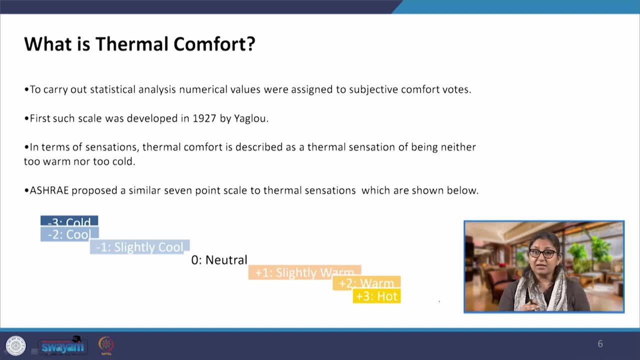 thermal comfort indices, thermal comfort index. and there they have. they have kind of devised kind of a scale, multiple different types of scales, to record how many people are feeling comfortable in the environment right now. So some are perception based scale, like Likert, simple scales where we, if we are comfortable, we will say we are neutral. 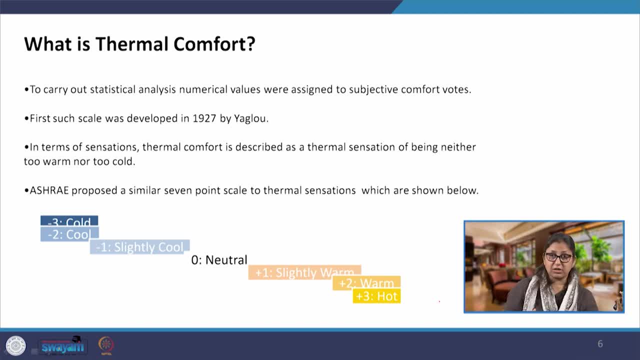 if we are feeling warm, hot or not, or cold or slightly cold. So this is, this is the range, this is the kind of scale that we have. There are also indices where we know exactly what affects thermal comfort and we know the quantitative value. So we know the temperature. 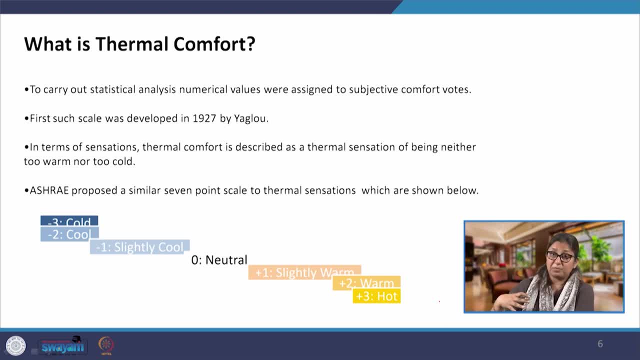 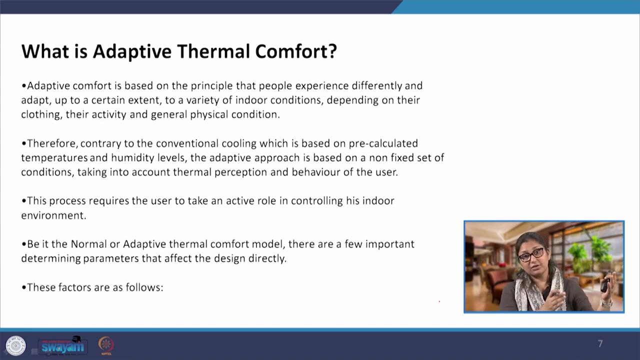 value. we know the relative humidity value and other factors which impact thermal comfort and we calculated to arrive at a thermal comfort number. So these are indices. different indices are there When we say that it varies from person to person be a fixed value. for a long time we had a fixed value. this is the range of thermal comfort. 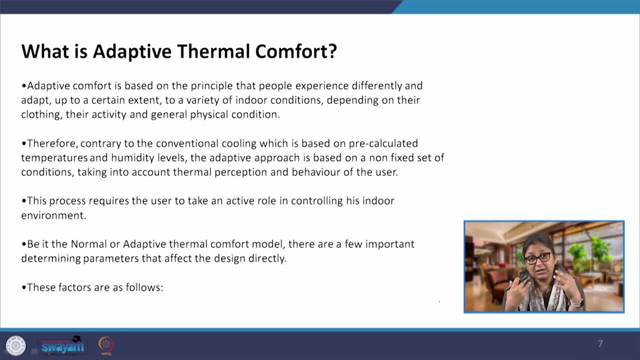 Now we also understand that the perception of thermal comfort, or how comfortable do we feel in a given set of conditions, varies from geographic region to region. this is dependent upon adaptability. So if we are living in India, we are relatively more comfortable at higher. 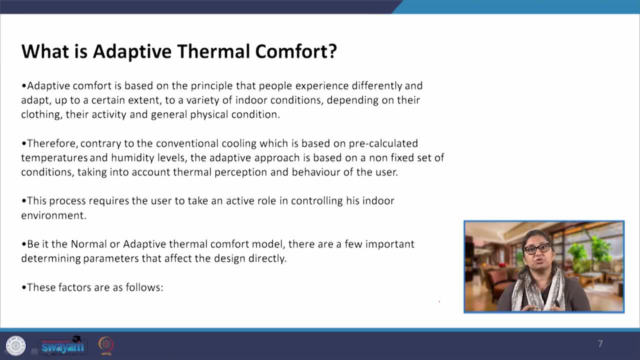 temperatures, at warmer temperatures, as compared to somebody living in Scandinavian countries or Nordic countries, where the average temperatures are much lower. So people adapt to the conditions around them, the environmental conditions around them, and that is what is exactly this adaptive thermal comfort tells us. So it varies. the comfortable zone, the comfort zone, varies for. 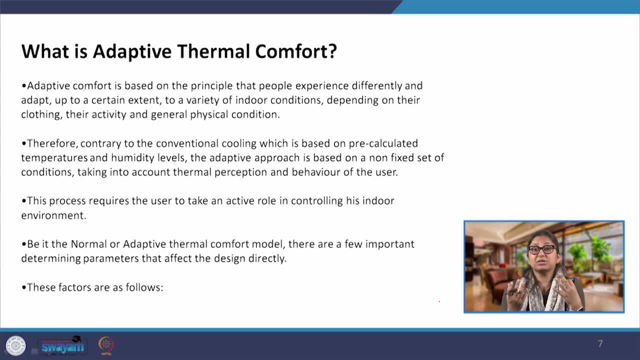 region to region and this, we, this different countries, have their own adaptive thermal comfort model where we see that how the comfort zone is shifting, it can also be a seasonal shifting. So since in India we are used to living specially in residential areas, we are used to living in unconditioned areas. 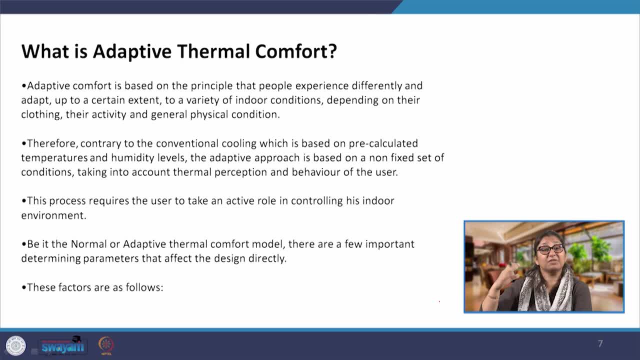 We do not condition our areas as the developed countries, the citizens in developed countries do. So we are more comfortable even at higher temperatures and also at lower temperatures, and adapt ourselves with clothing, with food, with activities. so this is all part of adaptive. 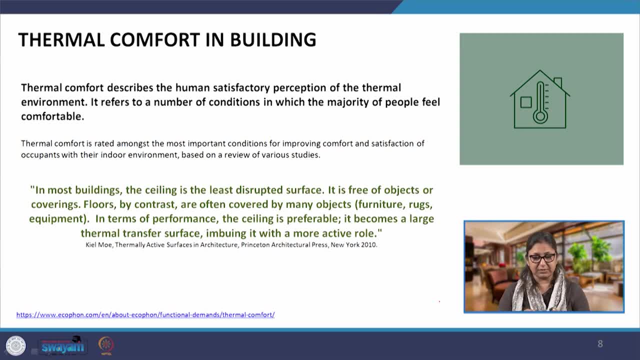 thermal comfort. Now coming to thermal comfort in buildings. so basically, thermal comfort describes the human satisfactory perception of the thermal environment And when we are talking about the buildings, we are talking about a lot of different parameters and factors which will contribute to the perception of thermal comfort. 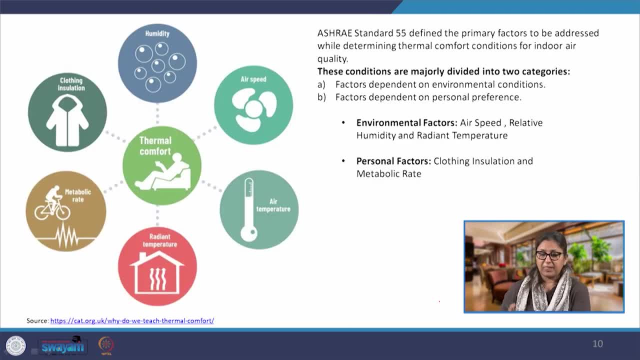 So what are these factors which affect thermal comfort? As per ASHRAE, there are two categories of factors. one is environmental factor, which is air speed, relative humidity and radiant temperature. We will come to each of these factors, but primarily we are talking about the temperature. 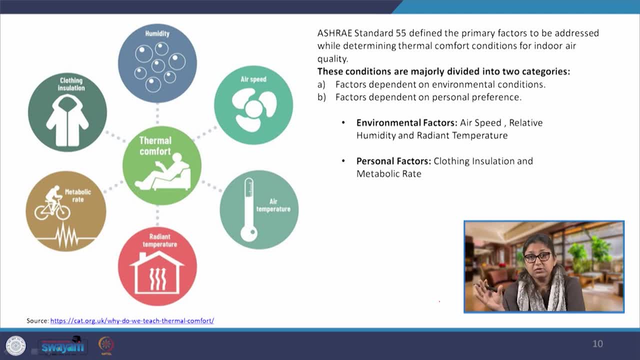 we are talking about the humidity and also the movement of air. Then we are talking about personal factors, which are clothing insulation. so how much clothing are we putting on? Because it provides us an insulation, and we know it. simply, we have seen when we want. 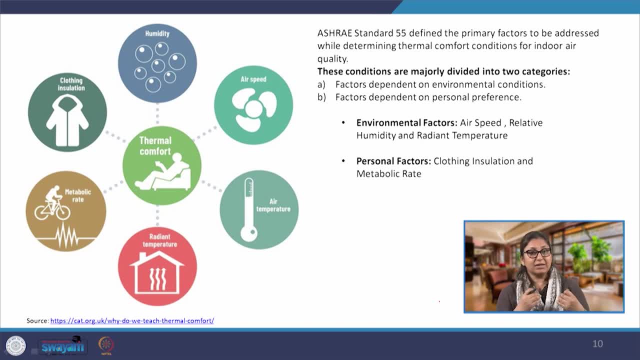 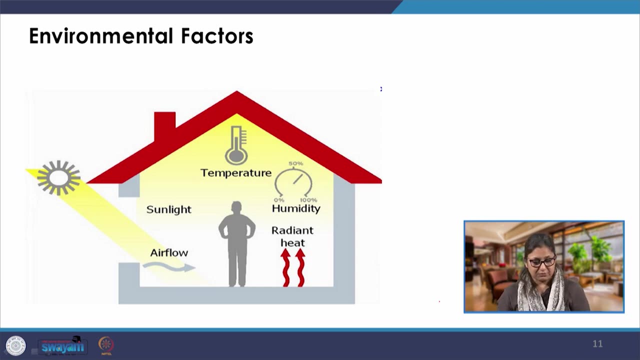 when we feel hot, so we provide less of clothing on our body, because it provides lesser insulation, so it allows heat to be dissipated faster. And the second one is metabolic rate. so, if so, we will come to all these factors one by one, but these are the five primary factors. 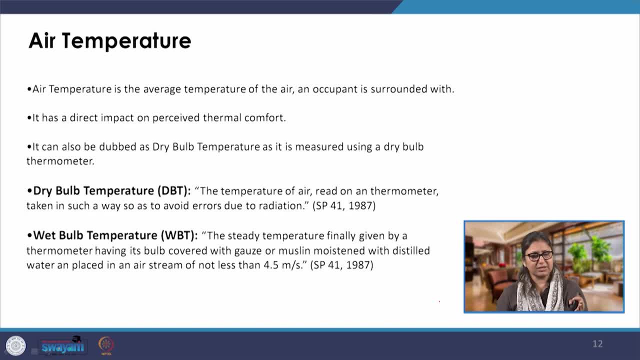 So if you are talking about environmental factors, first one is the temperature, the air temperature. So it is the average temperature of the air that the occupant is surrounded with. We have two temperatures. one is a dry bulb temperature, which is read on a regular thermometer. 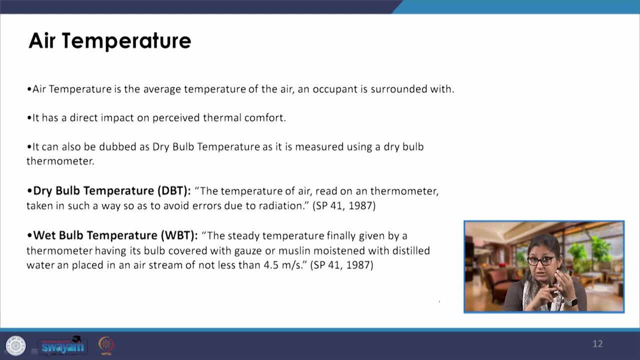 so now, this is not taking into account the effect of radiation or humidity that is present around. The second one is wet bulb temperature, which is the temperature which takes into account the evaporative cooling effect, which is reduced due to the presence of excessive moisture temperature. So we have dry bulb temperature, dbt, and we also have wbt, So both are measured. 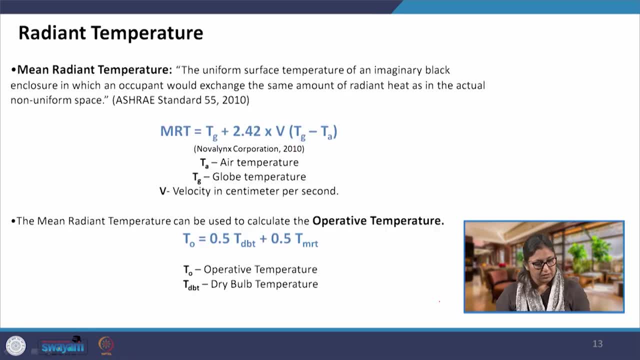 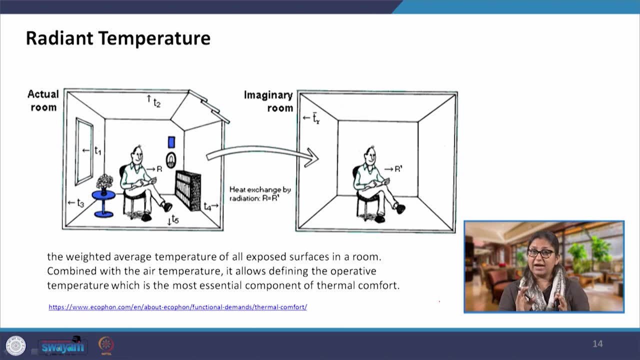 using thermometers, but different types of thermometers. Radiant temperature is, if I simply explain to you, it is the temperature at which the body radiates heat at the same pace, at the same rate as it is in a black body with a constant temperature. 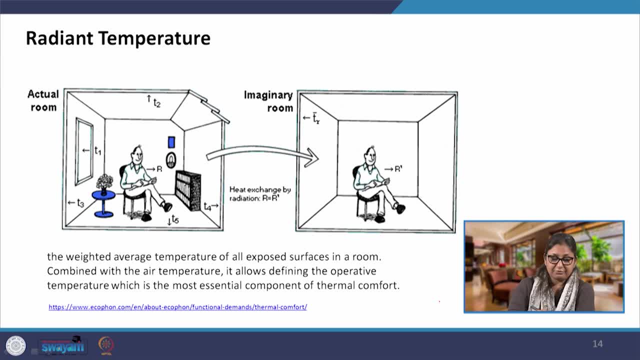 So basically, what we are talking about is, for example, we have a room, a person sitting in a room, which is this actual room. So we have different surfaces, we have a roof, we have a wall, we have a window. there might be radiation falling directly there might. 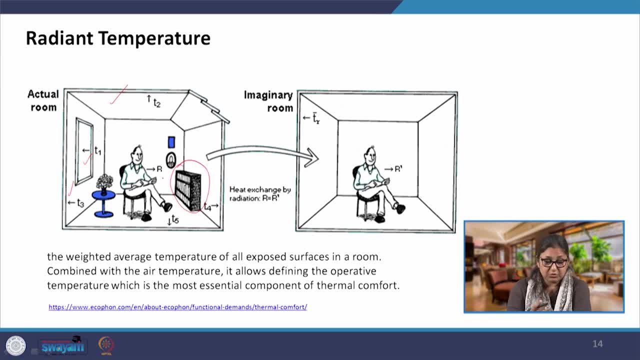 be some equipment which might be producing heat. So the human body is responding to all these radiations which are due to different temperatures of these surrounding bodies, but the human body is radiating at a rate which is r. Now, if it is extremely difficult, it is a complex scenario if we simplify it and we say that 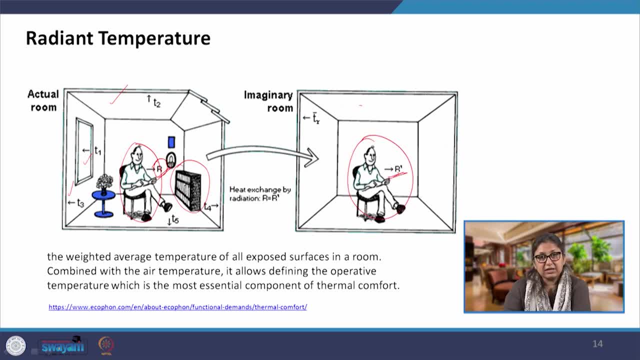 this human body, which is the same, is radiating at a rate r dash. So if all these surfaces around are at the same temperature, which can be the integration of all of them, and the resultant r and r dash remain the same, So r dash is same as r. 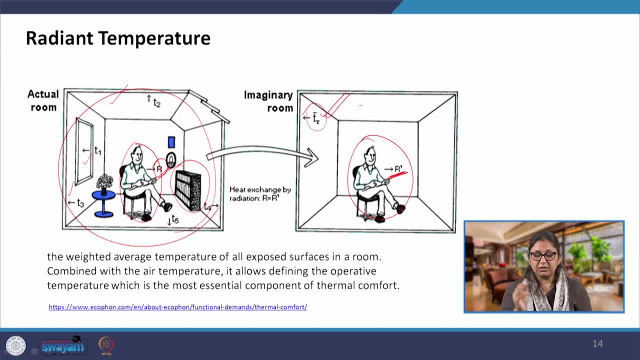 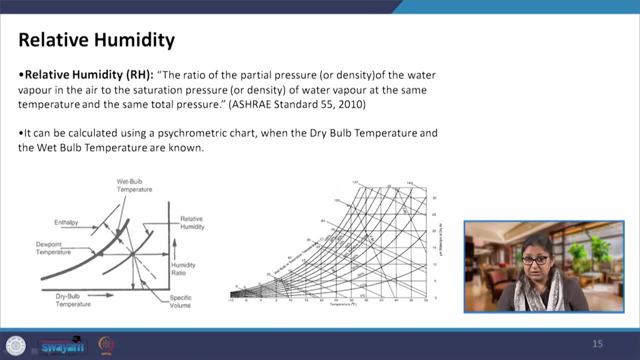 So this is the radiant temperature that we are talking about. So mean, radiant temperature is another factor that we talk about, and then relative humidity. Clearly, we understand relative humidity as a ratio of partial pressure or density of the water vapor in the air to the saturation pressure or density of water. 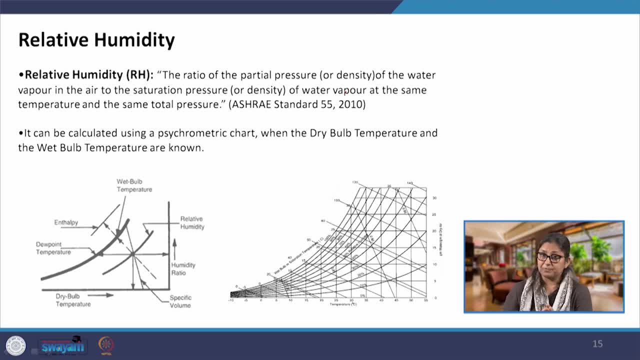 vapor at the same temperature and same total pressure. So basically, what we are talking about is when we have a higher relative humidity, which means the saturation level is higher, the capacity of air to absorb moisture or to take heat reduces. And when the air is drier, when there is less and less humidity, the humidity 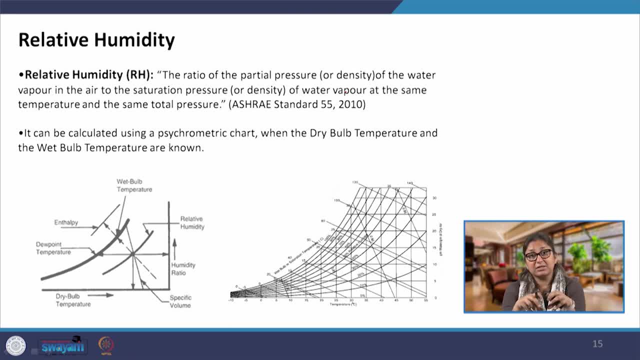 is becoming larger. So, basically, whenouts are less, and guys I am talking about depends on the вами, a denier, and the東 lesser amount of vapor, water vapor, present in it, it has a greater capacity to take moisture, to evaporate moisture and thereby taking away the heat. 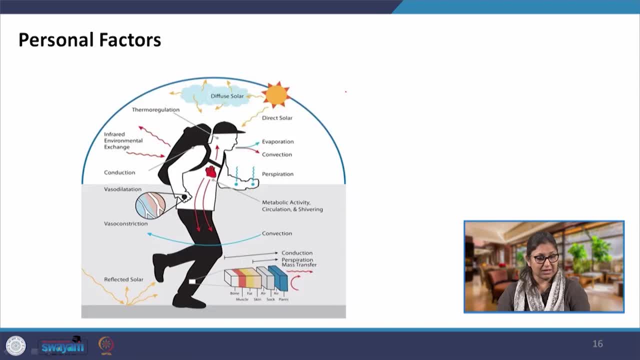 So this is the capacity that we are talking about when we say relative humidity. Now, coming to personal factors, we have a lot of internal processes that are going on in our body. we have evaporation, convection, perspiration is there. the body thermo regulates. 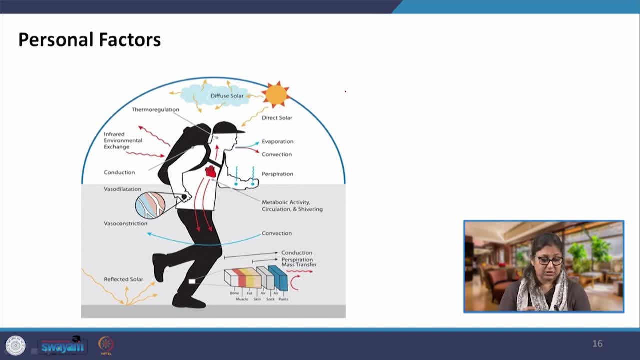 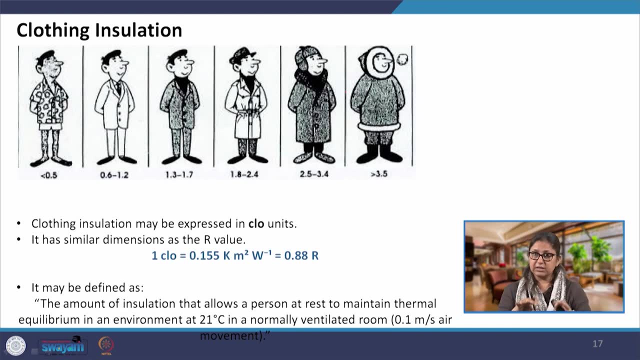 itself. So there are internal processes, such as vasodilation or vasoconstriction, which are happening inside the body But to be accounted for in the thermal comfort equation and the understanding of it. we are primarily looking at two factors. one is clothing insulation. 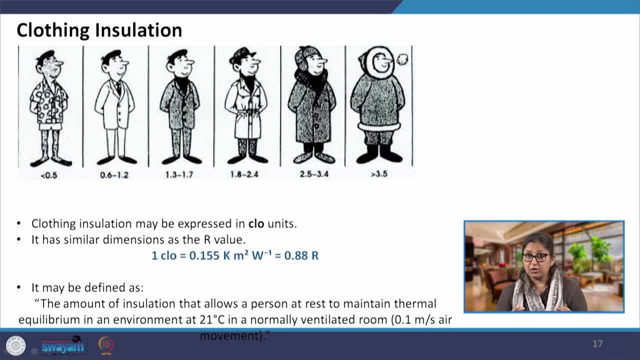 So higher is the amount of clothing that we put on, higher is the insulation due to clothing and it is expressed in a unit called Clo. So if you can see, here the Clo value is increasing From 0.5 here, from a very lightly dressed cotton clothes to heavy winter clothing. 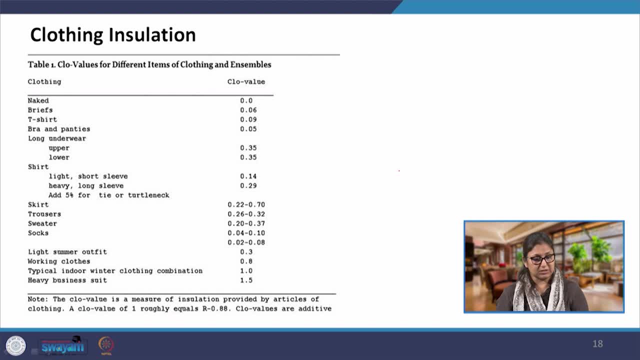 So this insulation is increasing, this Clo value is increasing and there are charts, there are numbers which are available for the clothing that we put on and the corresponding insulation value in Clo values. So the naked body is considered to be having a zero insulation because there is no insulation. 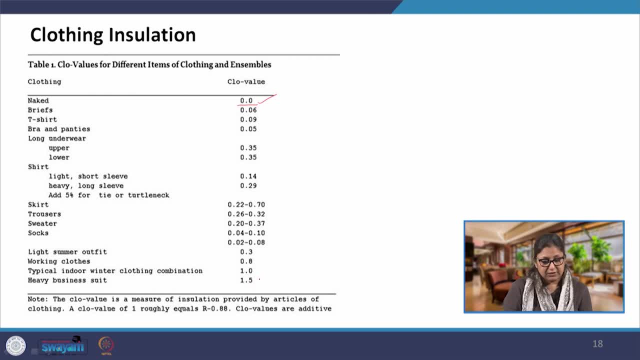 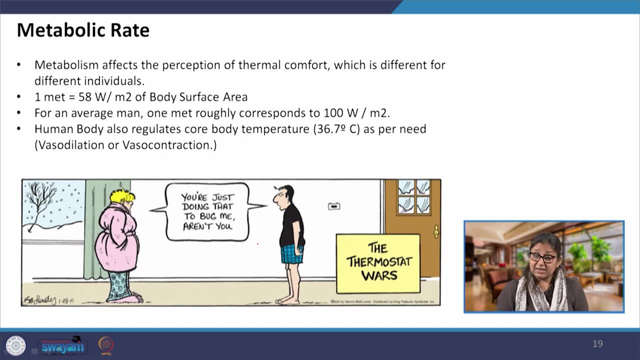 which is present, So that is provided, and then the heavy business suit and heavy winter clothing, so that has a higher value. Then the second thing is metabolic rate. our metabolic rate is dependent upon, again, a lot of factors. as I said, there are personal factors inside each human body and it varies from: 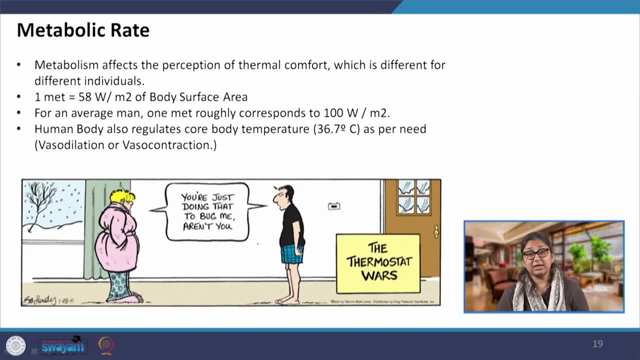 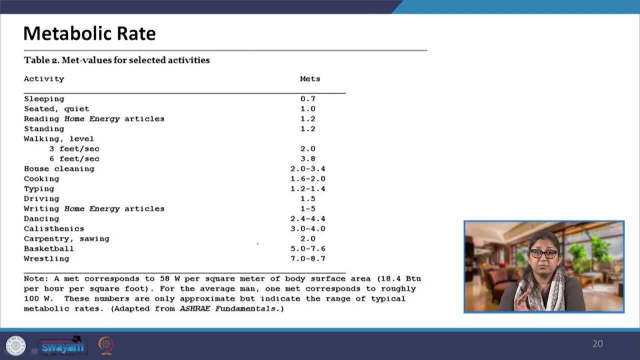 person to person. But largely what we understand is that it depends a lot on the activity that we are performing. So it depends a lot on the activity. So it depends a lot on the activity that we are performing. So we have, we generate, less amount of heat. when we say metabolic rate, it is the rate 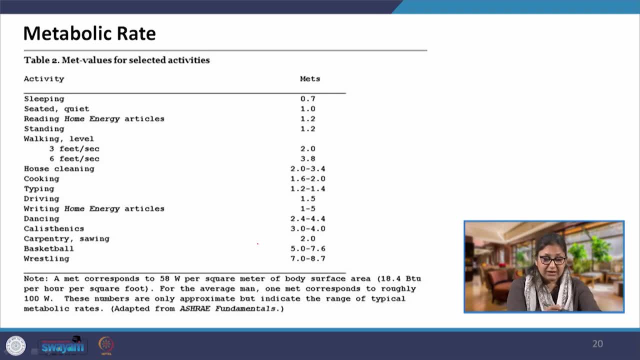 at which the body produces heat. So when we are sleeping, when our body is in a resting mode and there is no external activity being performed but only the internal processes, at that time also the body generates heat. But compare it with very heavy, high intensity activity. 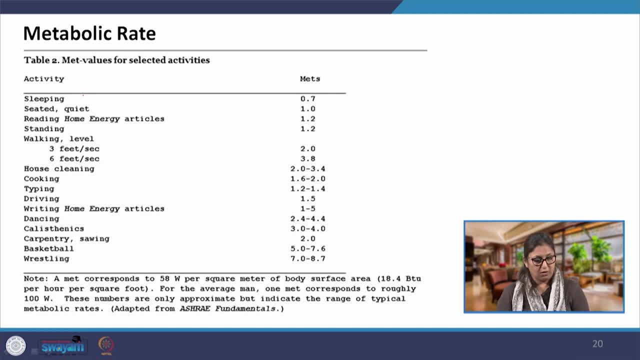 For example, wrestling. For example wrestling Or playing basketball or a very fast game, or working, for example- you know, intense working, like carpentry or sawing- so the metabolic rate increases. we perspire internally, the body also processes. So if we are running, then the body perspires, there is perspiration. that is happening and 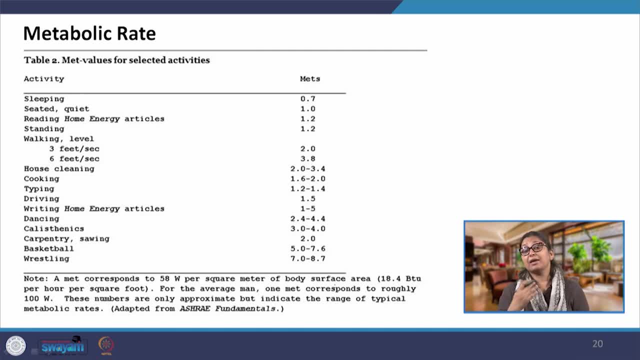 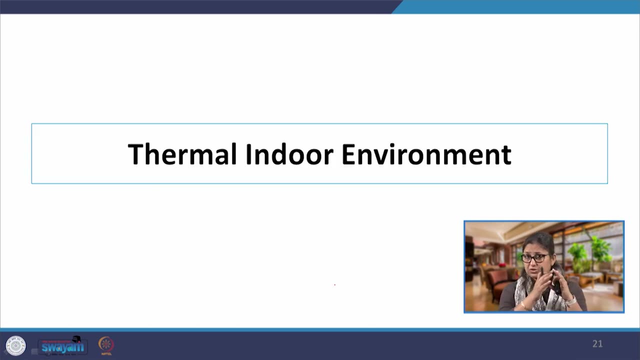 that we clearly understand that there is a high amount of heat. So metabolic rate is again a personal factor that is accounted for in the when we are trying to understand thermal comfort in buildings. Now, once we have understood all these environmental and personal factors, then we have to see that 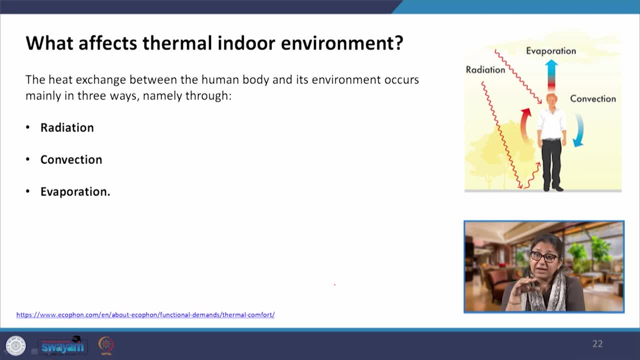 these are not the only factors which are going to affect the indoor environment. There are interactions with the external environment, That is, that are going to take place. So, primarily, there are three processes in which the heat exchange between the human body and its environment occurs: and this environment, which is the indoor environment, and the outdoor 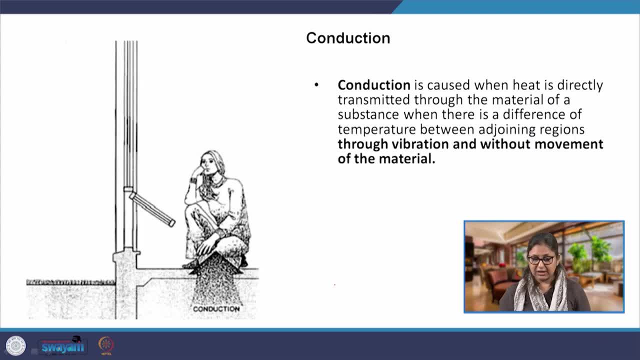 environment will occur. So we primarily have radiation convection and evaporation. So conduction is when the heat is directly transmitted. So these are simple processes. I am not going to go in detail over it yet. we are talking about the heat exchange. during the heat exchange. 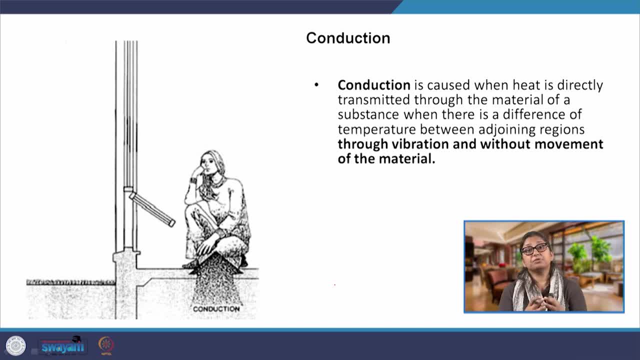 So we are talking about the heat exchange. So we are talking about the heat exchange during the heat exchange. So we are talking about the heat exchange. So that is the heat exchange due to two different materials coming in contact. that is conduction. 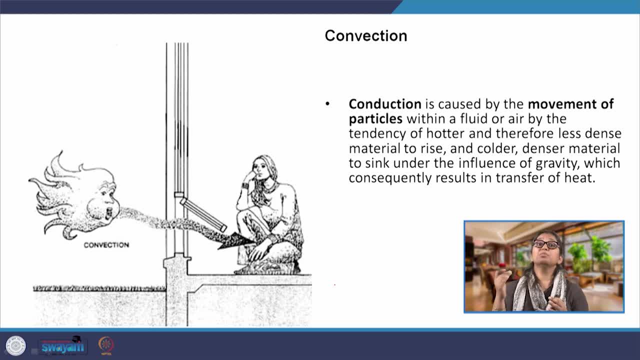 The second one is convection: when we know that it is due to the movement of particles and primarily when we are focusing on building. when we say convection, we are talking about ventilation, the movement of air. the convection is happening when the movement of air happens. 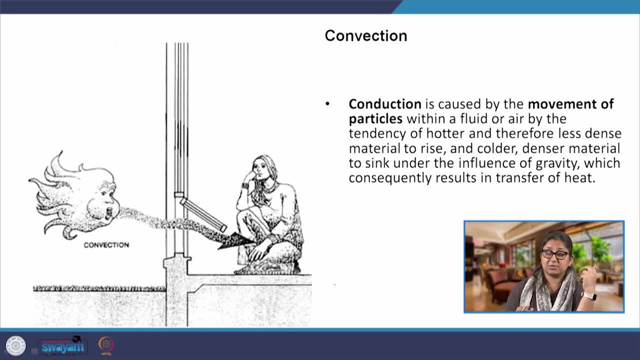 convection happens and that is how the heat exchange takes place. Every time I say heat exchange, It could be heat gain or heat loss. So when we are talking about warm tropical countries like India, we are primarily concerned with heat gain, because the outdoor temperature is often higher than the required. 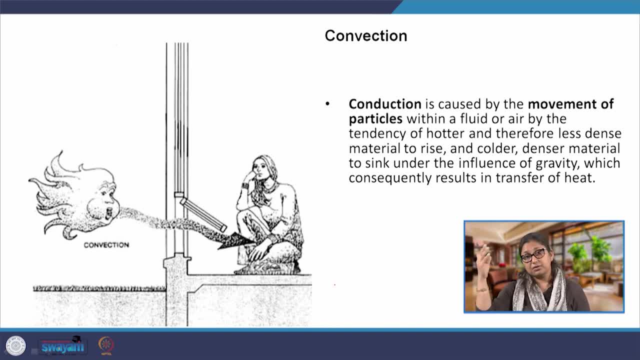 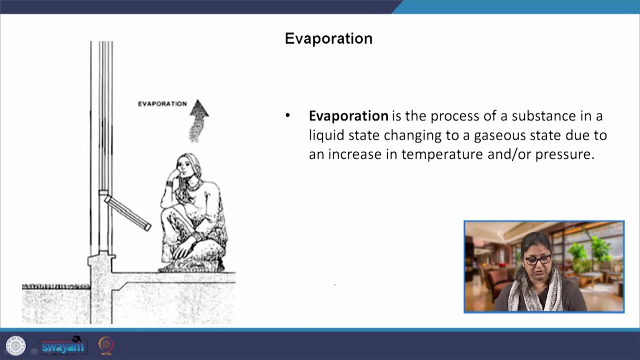 comfort temperatures. When we are talking about, for example, the extremely cold countries like the extreme northern parts or the extreme southern parts of the world, we are primarily talking about heat loss, because the average outdoor environment environmental temperature is lesser than the comfort temperature that we require. So this is convection. Then evaporation is the process. 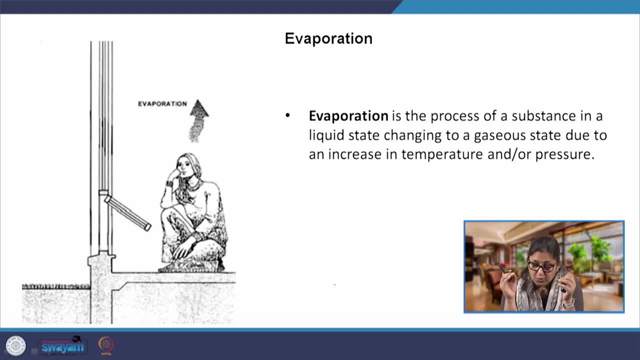 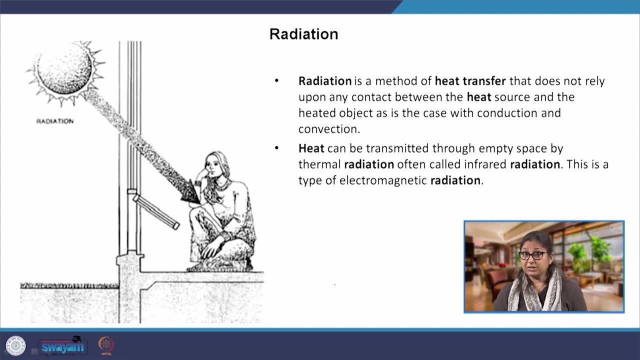 again, it is a heat exchange process where the state is changing from liquid to a gaseous state. So evaporation of water is often the activity that we are going to concern ourselves with when we are looking at thermal completamente comfort in building. and the last one is radiation, which is extremely important because the buildings 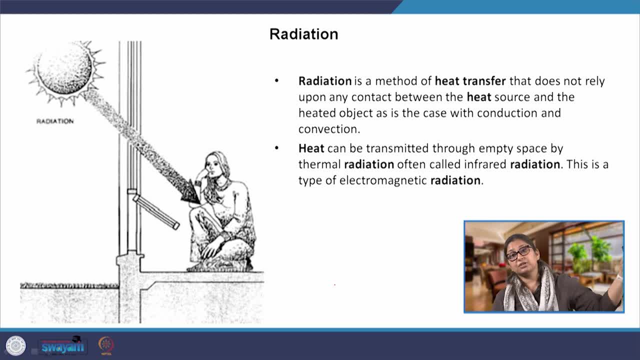 get heated primarily due to the heat received from sun, the solar radiation. So sun brings in a lot of heat. now, in certain scenarios, for example the warm tropical climate, we will not need to bring in all that radiation inside, but that is again not throughout the 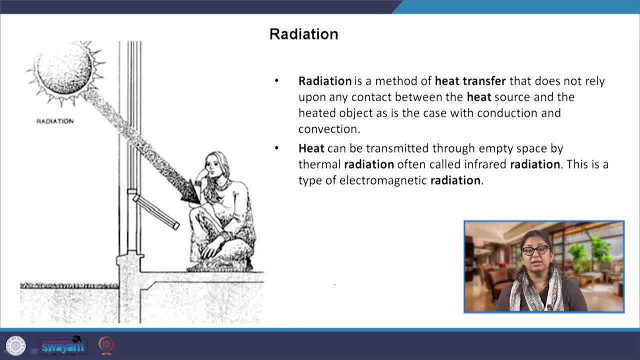 year. So in extreme winters we may want to bring sun inside and in extreme summers we may want to cut off this solar radiation, while in extremely cold countries we may want sun throughout the year to be brought inside. Now, how do we do? that is what we have to understand: these processes, these fundamentals. 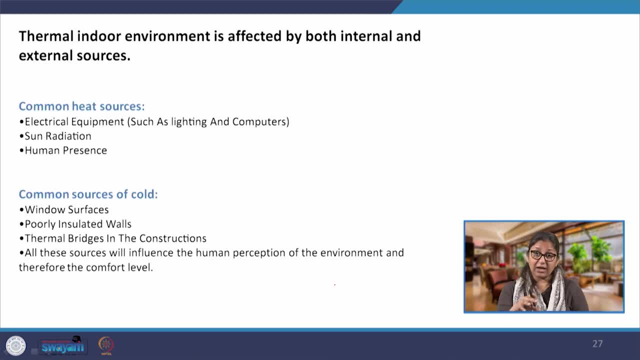 only tell us that what all is possible. but what we have to now see further ahead is: how do we really achieve the thermal comfort What happens inside the building, through design as well as construction. Now, if we look at the sources, both internal and external, the heat sources and sources, 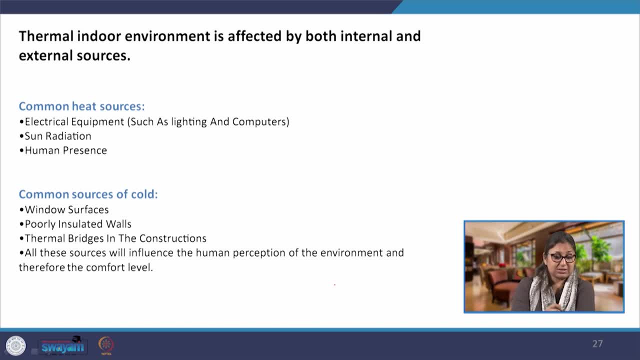 of cold. So then we see that in the building, as I have just said, solar radiation is the primary source of heat for buildings. In addition to that, we have different equipments and appliances which produce heat. we get heat from the, from the light, artificial lighting, because all luminaries, they have a fraction of this energy which 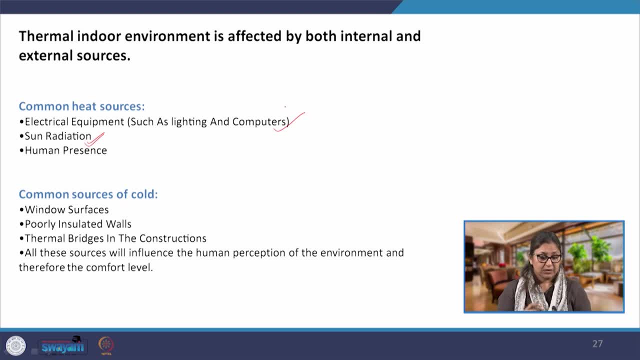 is also converted into heat, besides the light that it gives us. So we have lighting fixtures, we have equipment such as computers, we have many other equipments that are going to be inside the building and they produce heat. they add heat into the building. this is process heat. 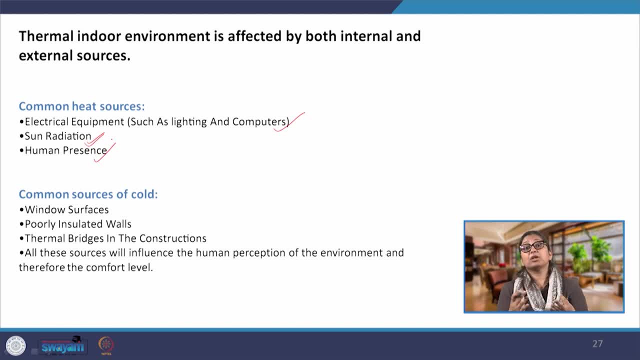 And then we also have human presence. so we just have seen the metabolic rate. So if there are only few people sitting in the room- say 4 or 5,, then the amount of heat that they add into the environment is lower. and compare it with 100 people sitting. 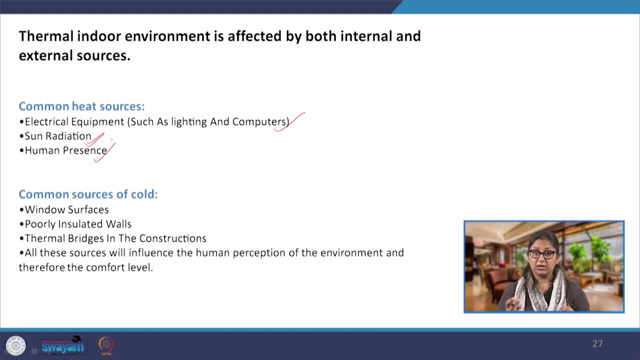 in one room. suddenly the room becomes very hot. we are not even talking about the carbon dioxide that is exhaled by the people, but we are primarily talking about the heat that is released into the environment. So when it is extremely cold, we tend to huddle together animals. in general, you would. 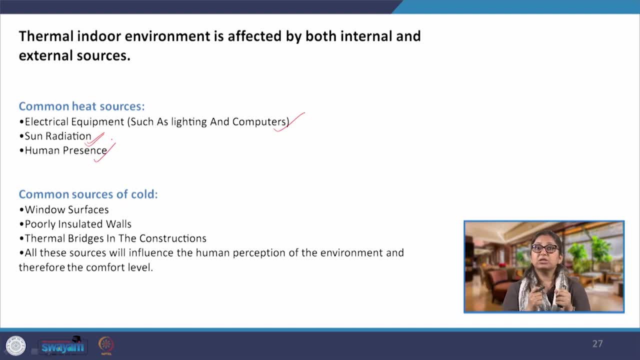 see that when it is extremely cold. So we tend to huddle together animals in general. you would see that when it is extremely cold they would come very close to each other because they are giving heat to each other and they are also conserving heat by reducing the surface area. 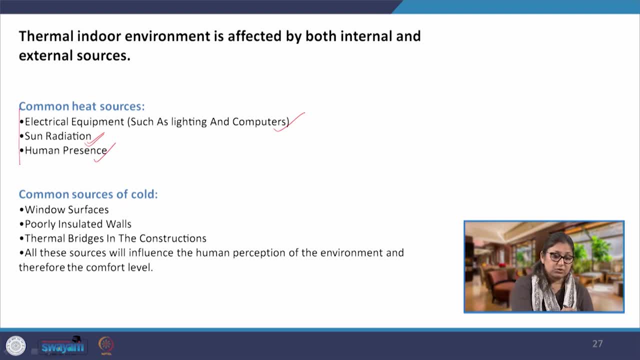 So all these things, we are going to see further, but these are the common sources of heat that we have to tackle and, if we have, we are talking about cold countries. we are talking about these sources of cold. So we are talking about different surfaces, not just window surfaces, but all the surfaces. 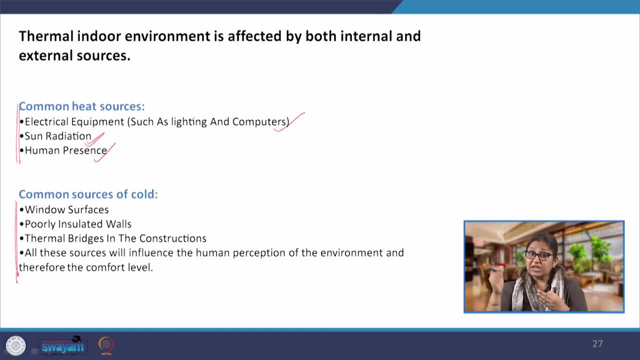 of this building, which can exchange heat. due to condensation, Any body which is at a higher temperature will radiate heat to another body or environment which is at a lower temperature. So we are talking about all surfaces: window surfaces, wall surfaces, roof surfaces and. 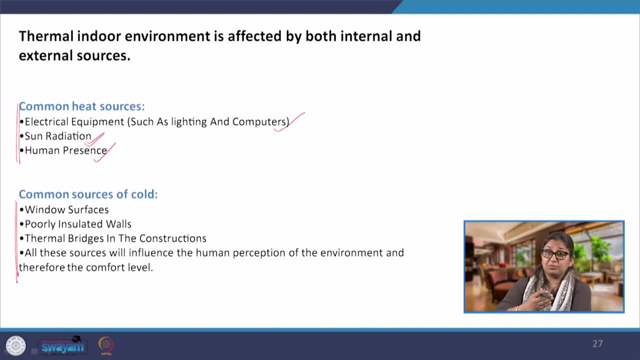 to reduce that, we may be needing to have insulation provided so that less heat exchange is happening through different processes. Then we are also talking about the leaks and bridges throughout the building, So thermal bridges in the construction, which are the common sources of heat loss in buildings. 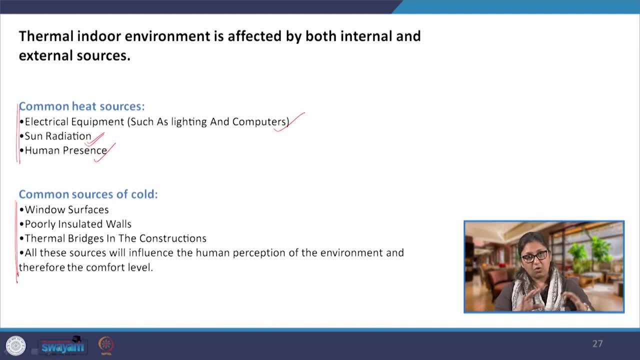 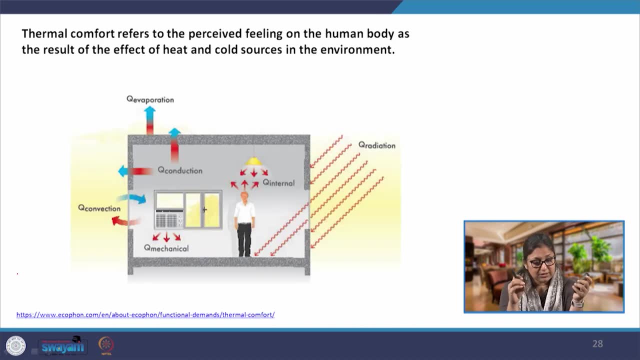 Now, all these sources, whether they are of heat or cold, they have to be tackled when we are designing buildings if we want to reduce the energy consumption. This is something that we have to understand, that how this whole understanding of thermal comfort is translated into GHG emissions. 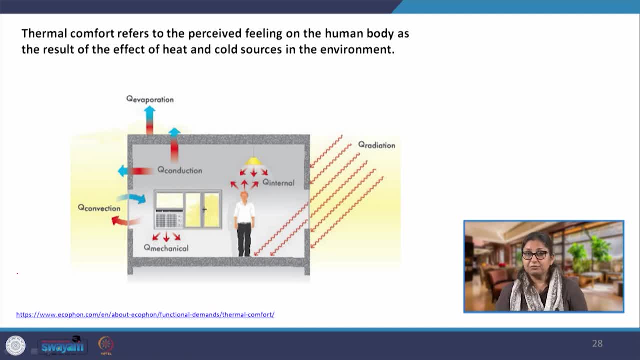 Now, if there is less comfort, which is in inside the building, or the building is not comfortable, Then what will I need to do today? we will add air conditioning, or we will add fans, or we will add artificial lighting. In case of thermal comfort, we will add HVAC. whether we will heat the building or we will 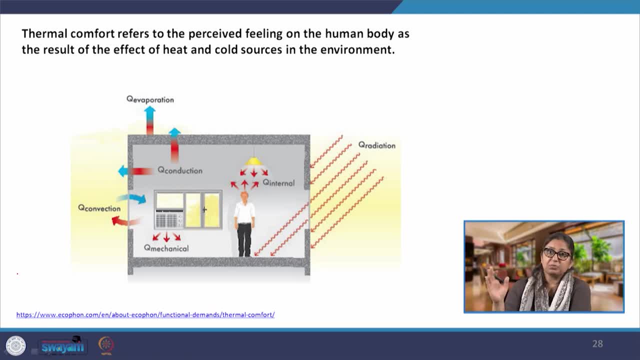 ventilate the building or we will cool the building. either of the three processes will be happening there mechanically. And when we have to do all that mechanically, then we will be adding electricity, or we will be consuming electricity to extract the heat out of the building or to provide heat into. 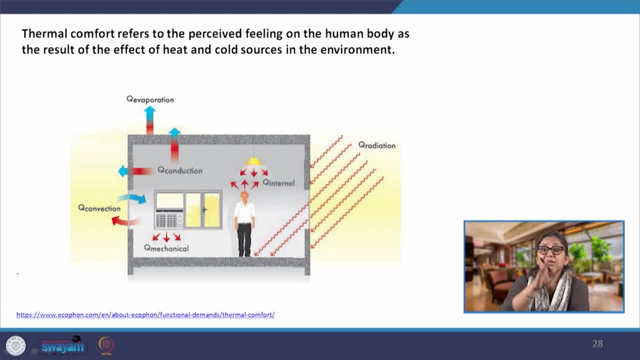 the building. Now this thermal comfort is directly translating into energy consumption, And the moment we see that the building needs electricity to maintain comfort, we are directly talking about scope 2 emissions. Now this link has to be directly clear. if the building is comfortable, there is less. 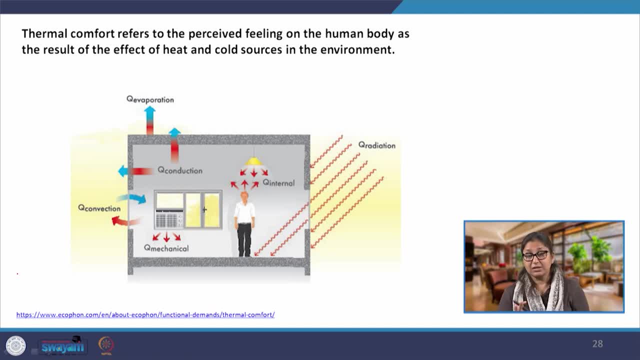 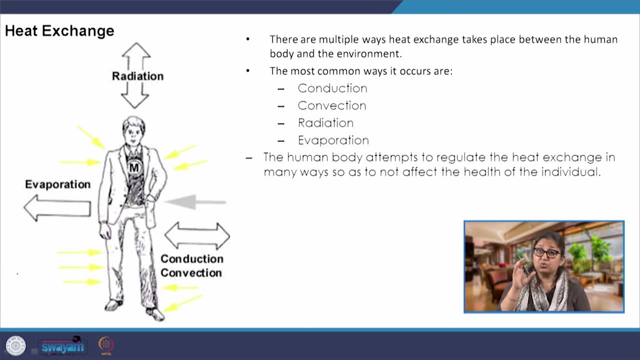 of scope 2 emission, GHG emission- that is going to be there: Less energy consumption, less GHG emissions, And so what we need to do is we need to reduce the amount of energy that is required for conditioning the environment and make it passively cool. 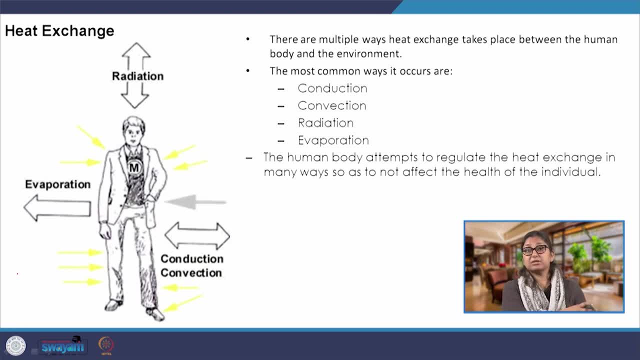 The other thing that we can also do is personal factors. Now, activity we cannot control, because if it is an office building and people tend to sit on their seats for a long time, Their metabolic rates are going to go down And that means their muscle activity. 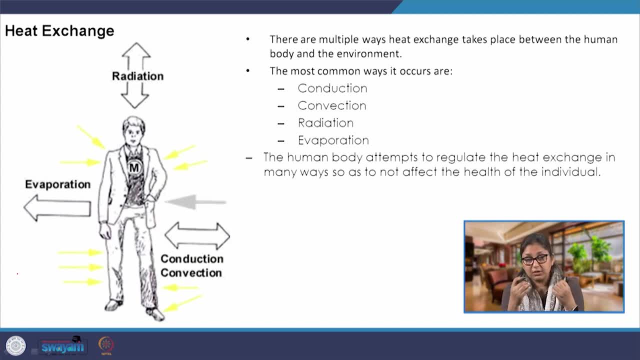 Nobody wants that right to be lower. the amount of heat that they produce are going to be lower In extreme cold climates, in extreme cold season. we cannot ask people to start indulging in high intensity activities. we cannot ask them to start running and jogging around that. 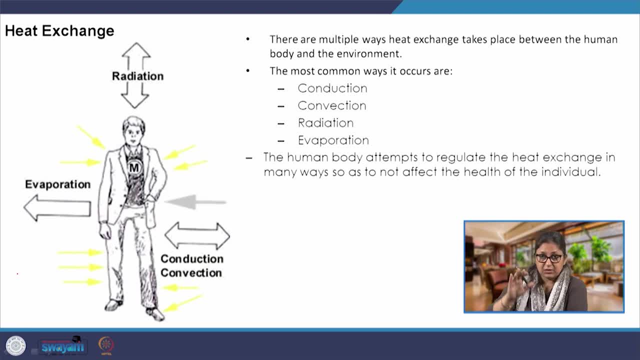 is not possible, So the activity part is separate. there is no impact on it. but what we can influence through behavioral change and the requirements is the acceptance of kind of clothing that they put on. For example, in corporate offices the commonly accepted attire, even in extreme summers, is: 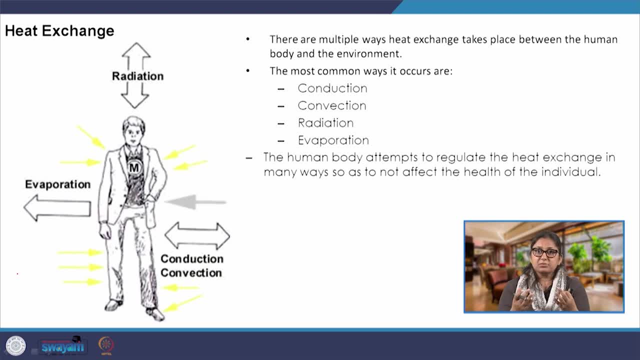 a coat, a blazer. Now, it adds a lot of insulation to the human body and if you have to put on a blazer or a coat, we will need to add extra electricity, extra cooling into the space. because the metabolic rate is going to be higher, there is more amount of cooling that is required to keep. 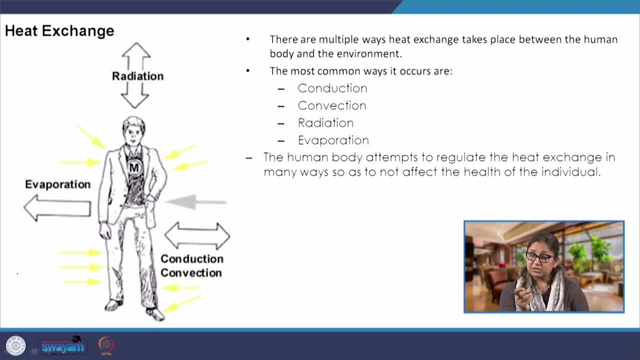 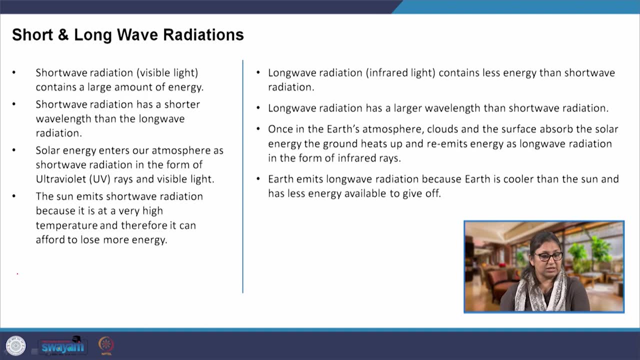 the person comfortable, So these behavioral changes can also make the requirement as lesser and eventually the GHG emissions. Another thing that we have to understand about this whole process, or different processes by which heat exchange takes place, is the capacity of this hard surface. most of the 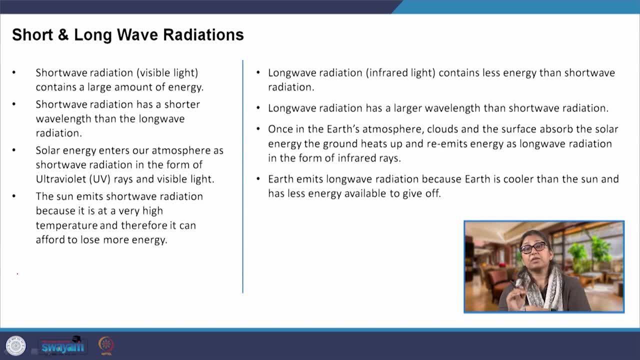 materials of which the building is constructed, So we have to allow them to absorb heat and then to re-radiate it at a later time, and this is where we are talking about short and long wave radiations. Now, short wave radiations are the radiations that are received from sun. they travel a.